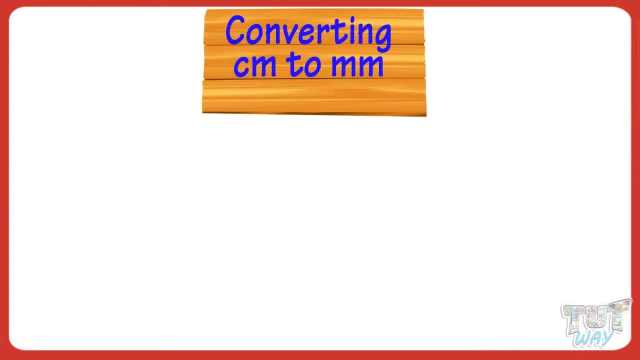 centimeters to millimeters. One centimeter equals 10 millimeters, So whenever you have to convert a unit into a millimeter, you have to convert it into a millimeter. So let's learn how to convert centimeters to millimeters. You will multiply them with 10.. Let's convert. 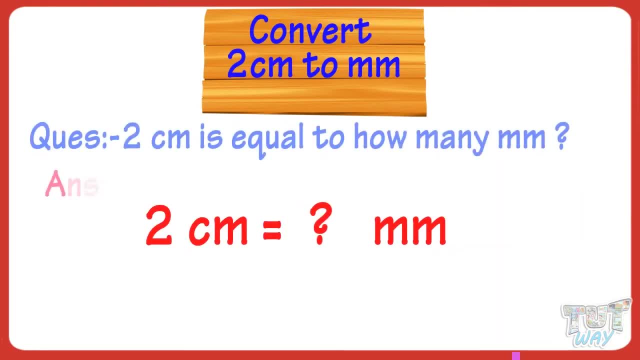 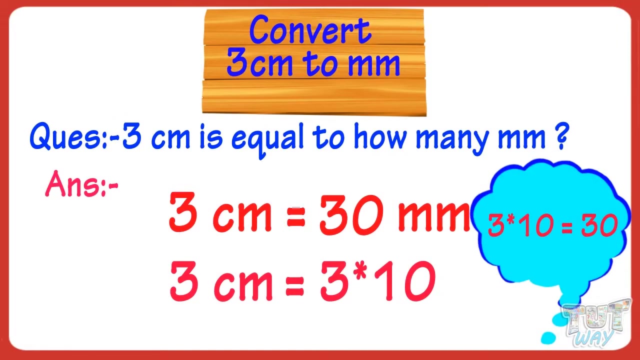 two centimeters to millimeters. Multiply two with 10.. Two multiplied by 10 equals 20.. So two centimeters equals 20 millimeters. Let's convert three centimeters to millimeters. Three multiplies by ten, we get thirty. So three centimeters equals thirty millimeters. So we 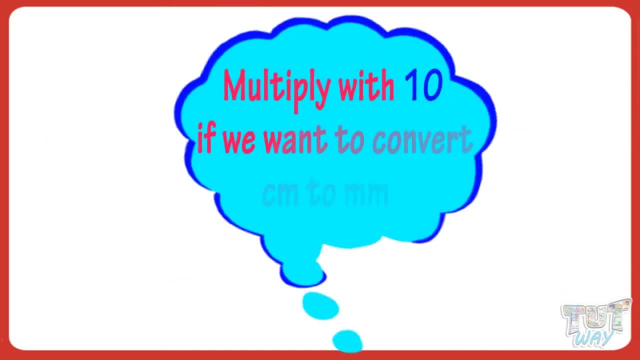 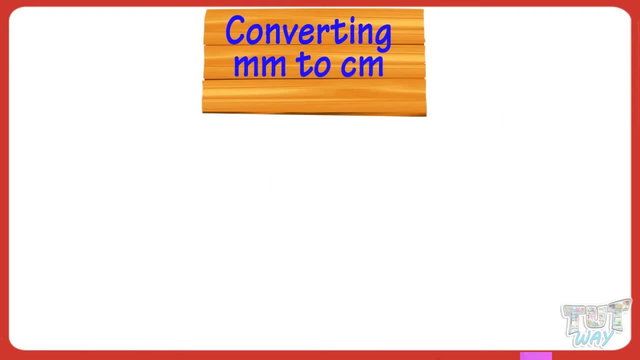 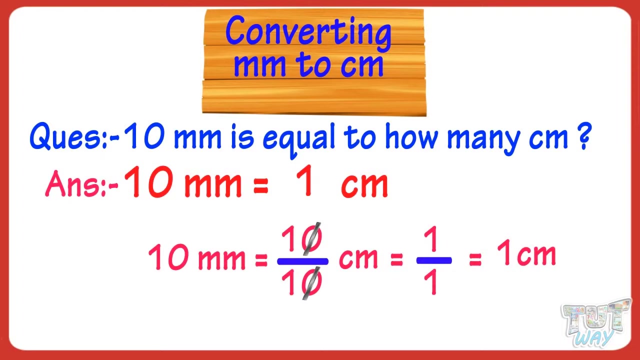 multiply with ten if we want to convert centimeters to millimeters. Now let's learn converting millimeters to centimeters. 10 millimeters is equal to how many centimeters 10 millimeters equals 10 millimeters. 10 divided by 10 centimeters, 10 divided by 10, we get 1.. So 10 millimeters equals 1 centimeter. 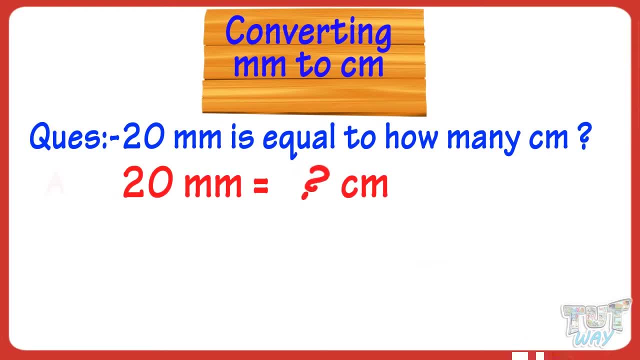 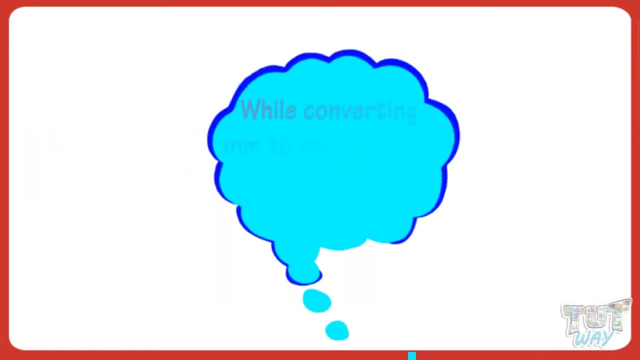 20 millimeters is equal to how many centimeters? 20 divided by 10 equals 2.. So 20 millimeters equals 2 centimeters. So, kids, when we have to convert back millimeters to centimeters, we divide by 10.. Now let's learn converting meters to centimeters. 1 meter equals 100. 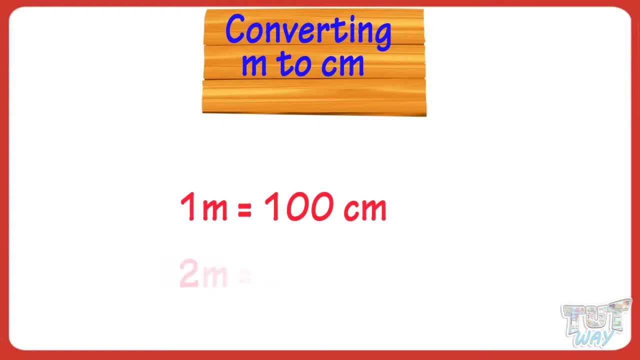 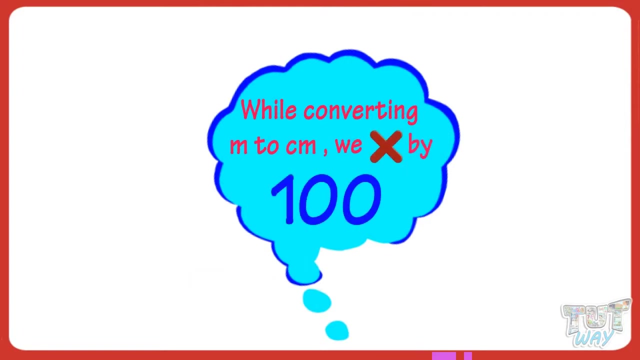 centimeters. So 2 meters equals 200 centimeters. That is, we multiply with 100.. 3 meters will be equal to how many centimeters. It will be 3 multiplied with 100. So we get 300 centimeters. So, kids, we multiply with 100 if we want to convert meters to centimeters. 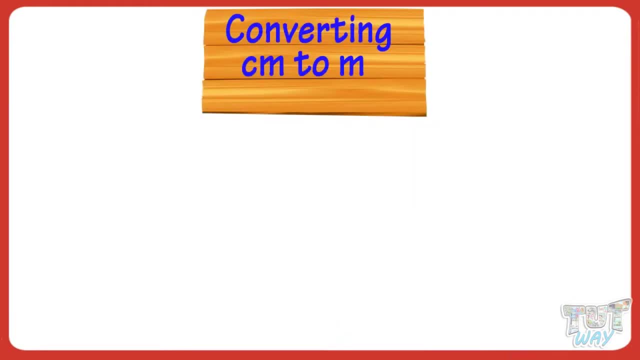 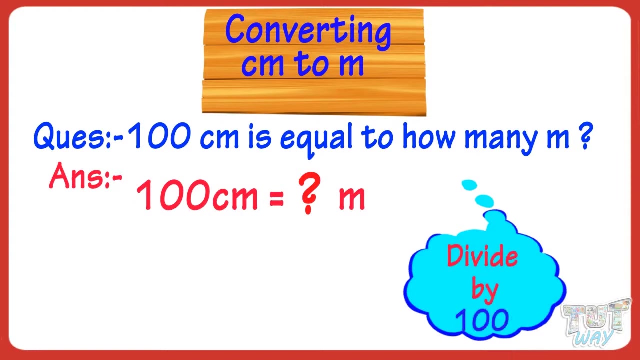 Now let's learn converting centimeters to meters. 100 centimeters is equal to how many meters? For converting centimeters to meter, we divide by 100.. As 1 meter equals 100 centimeters, So 100 centimeters equals 100 divided by. 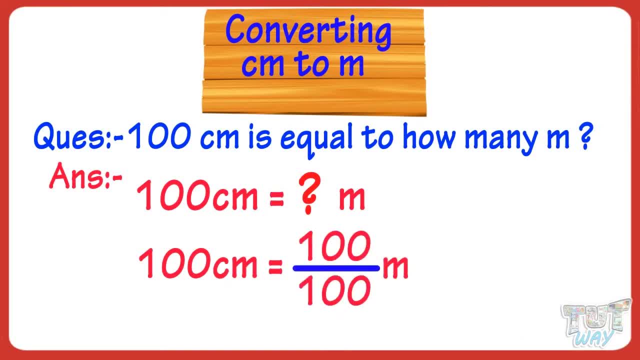 100 meters. 100 divided by 100 equals 1.. So 100 centimeters equals 1 meter. 200 centimeters is equal to how many meters? For converting centimeters to meter we know, we divide by 100.. So 200 centimeters equals 200 divided. 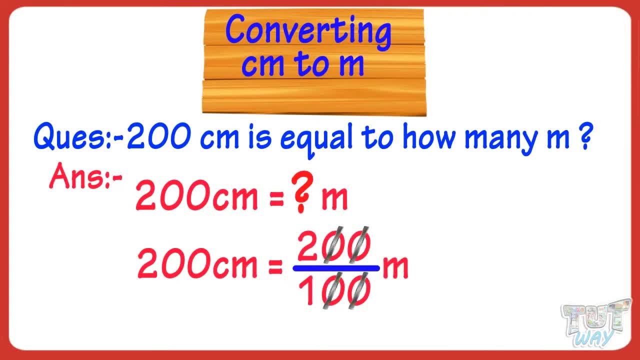 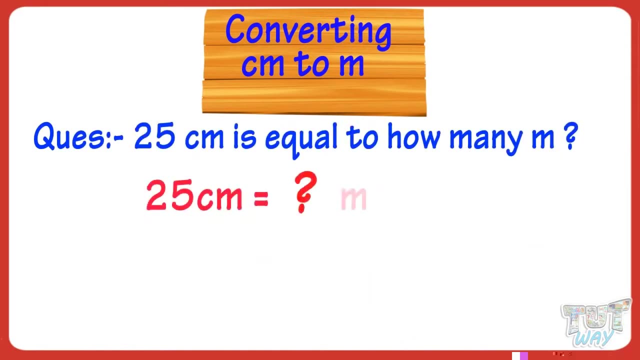 by 100 meters. 200 divided by 100 equals 2.. So 200 centimeters equals 2 meters. 25 centimeters is equal to how many meters We know. we divide by 100, while converting centimeters to meter. 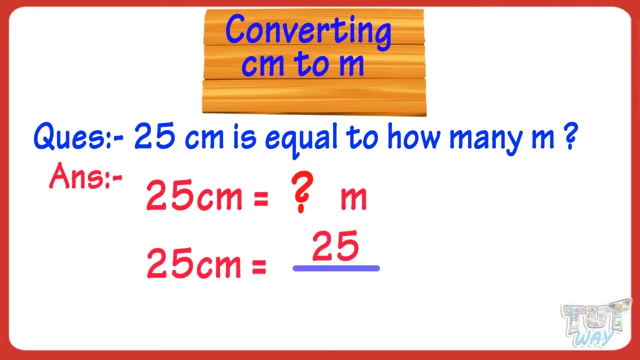 So 25 centimeters equals 25 divided by 100.. 5 multiplied by 1 meter, 1, by arbitration, имеет 2 meters, 100 meters. Cutting two zeros and putting decimal after two digits, from right we get. 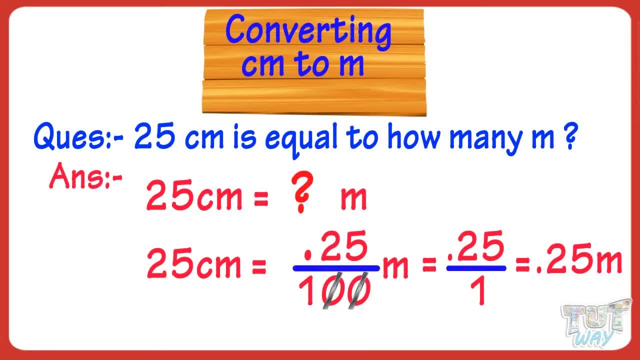 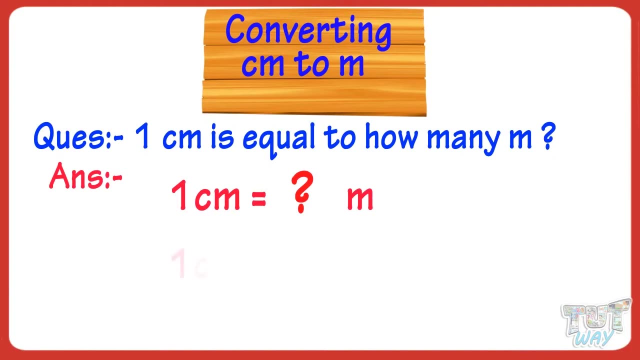 0.25.. So 25 centimeters equals 0.25 meters. One centimeter is equal to how many meters? One centimeter equals 1 divided by 100 meters. So cut two zeros. we have to put decimal. 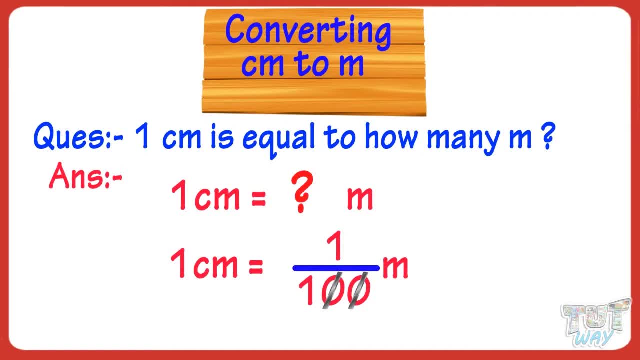 after two digits from right, But as there is only one digit, so we put one zero on left and insert decimal, So we get 0.01.. So one centimeter equals 0.01 meters. Now let's learn converting kilometers to meters. 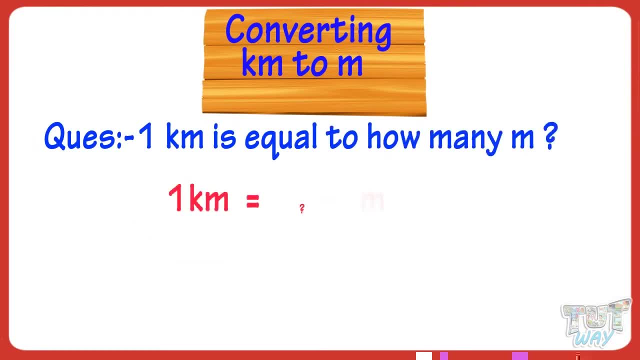 1 kilometer is equal to how many meters? 1 kilometer equals 1 multiplied by 1,000 meters, That is, we multiply by 1,000.. We want to convert kilometers to meters, So 1 kilometer equals 1,000 meters. 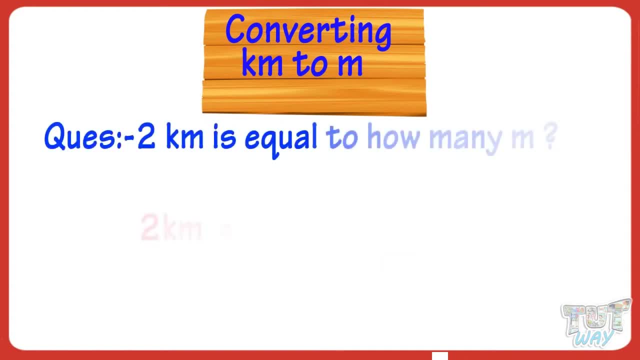 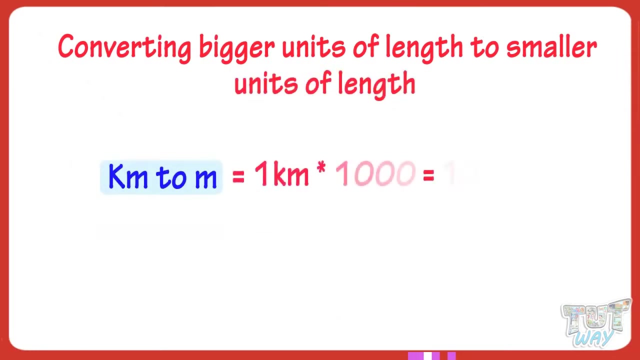 2 kilometers equals how many meters? Multiplying 2 by 1,000, we get 2,000.. So 2 kilometers equals 2,000 meters. Kids, whenever we convert bigger units to smaller units, like kilometers to meters, meters to centimeters, 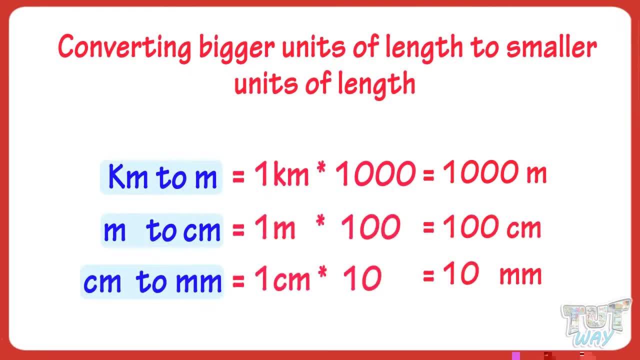 centimeters to millimeters, we multiply. When we convert kilometers to meters, we multiply by 1,000.. When we convert meters to centimeters, we multiply by 100.. When we convert centimeters to millimeters, we multiply by 10.. 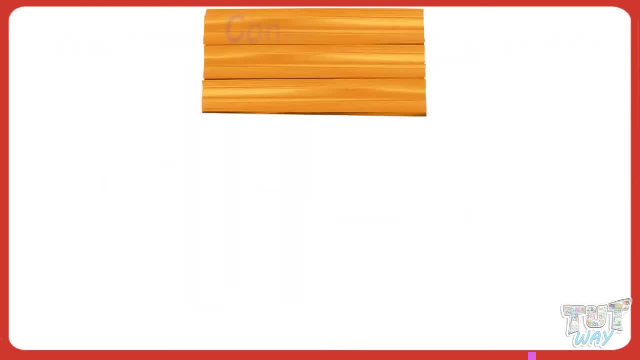 Now let's learn converting meters to kilometers, That is, smaller unit to bigger unit. 1 kilometer equals 1 multiplied by 1,000.. And whenever we convert smaller unit to bigger unit, we divide 3,000 meters equals how many kilometers? 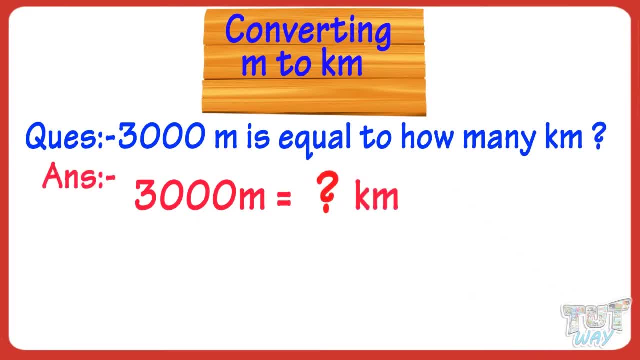 We will be dividing by 1,000.. So 3,000 meters equals 3,000 divided by 1,000 kilometers, Cutting three zeros, we get 3.. So 3,000 meters equals 3,000 kilometers. 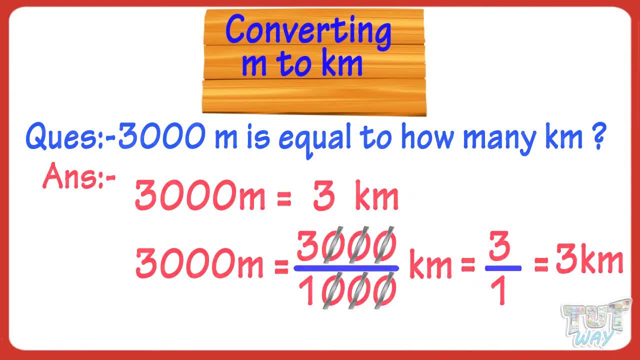 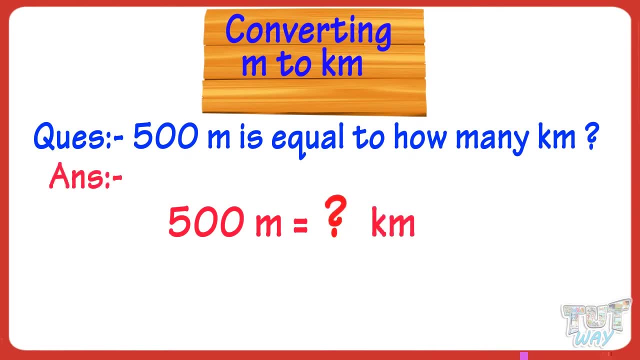 500 meters equals 3,000 kilometers. 500 meters equals how many kilometers We will divide by 1,000.. So 500 divided by 1,000 kilometers, Cutting three zeros, we put decimal after three digits, from right.